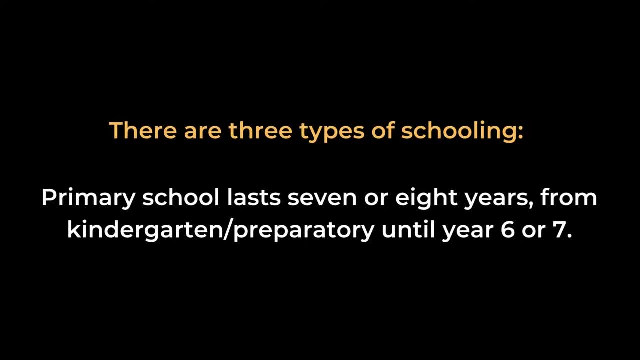 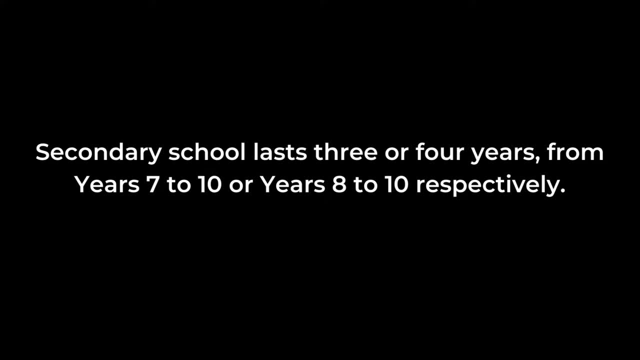 Primary school lasts 7 or 8 years, from kindergarten or preparatory until Year 6 or 7.. Secondary school lasts 3 or 4 years, from Year 7 to 10 or Years 8 to 10 respectively. Senior Secondary School- Years 11 and 12,- is a two-year programme. 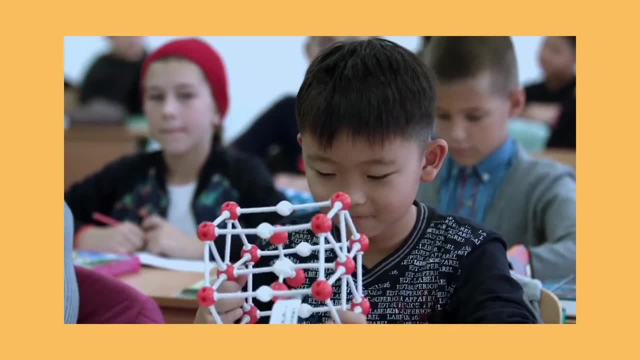 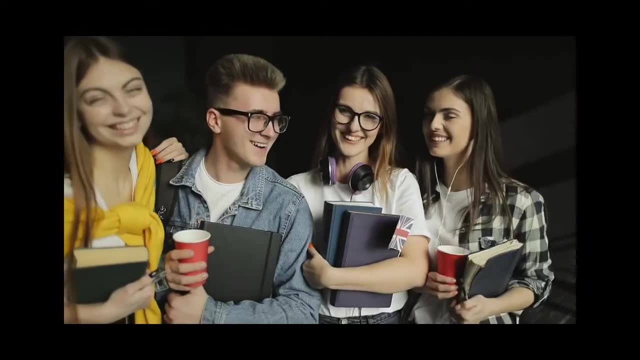 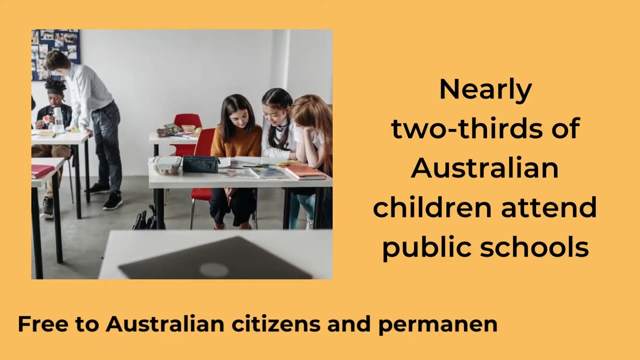 Senior Secondary School- Years 11 and 12, is a two-year programme. Government-funded public schools, as well as private schools such as Catholic and Independent Schools, provide primary, secondary and senior secondary education. Nearly two-thirds of Australian children attend public schools, which are free to Australian citizens and permanent residents and attended by nearly two-thirds of the children in Australia. Vocational Education. Vocational Education and Training VET is artistic and 두�iagno benefici. Vocational Education Vetos. Vocational Education VET are essential skills. Vocational Education VET is educational skills and secondary security. 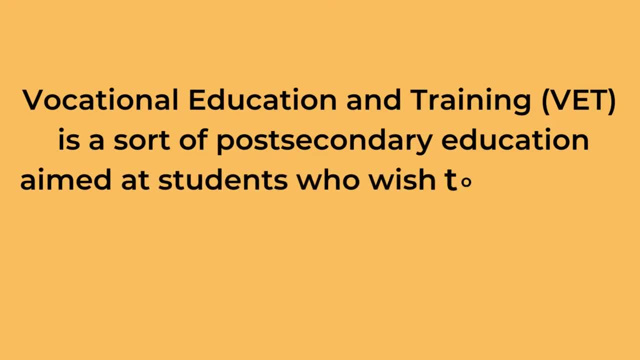 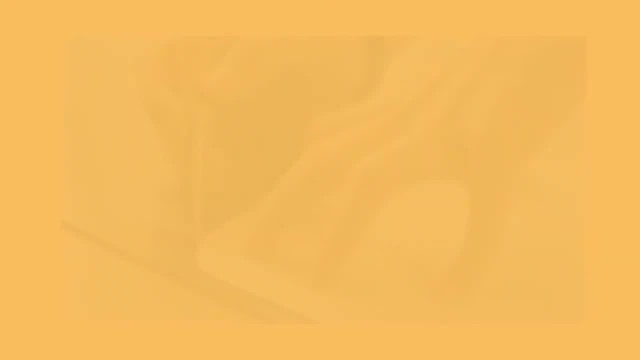 is a sort of post-secondary education aimed at students who wish to enter the workforce right away and work in jobs that do not need a university diploma. VETs offer courses and training for semi-skilled, skilled trade and paraprofessional vocations. 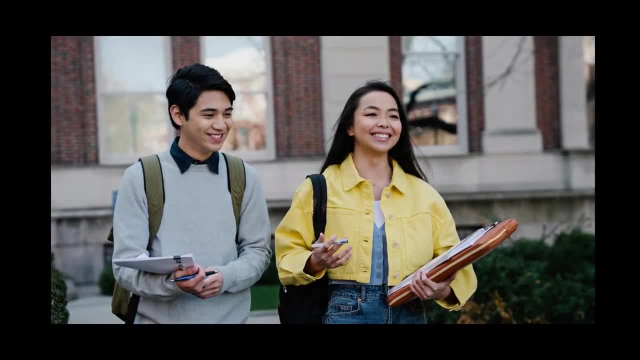 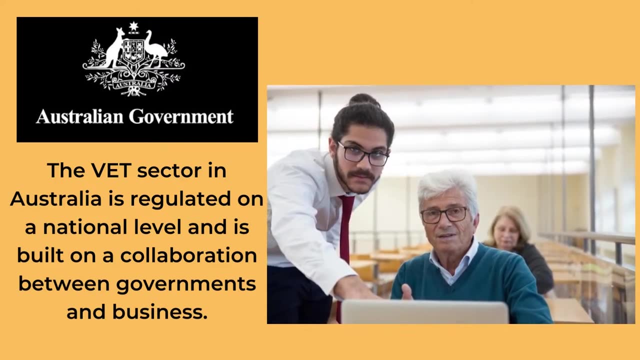 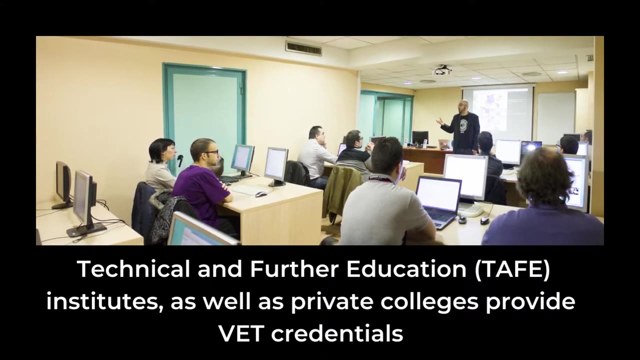 providing a more hands-on alternative to university education. The VET sector in Australia is regulated on a national level and is built on a collaboration between governments and business. Government colleges, known as Technical and Further Education, TAFE institutes, as well as private colleges, provide VET credentials. 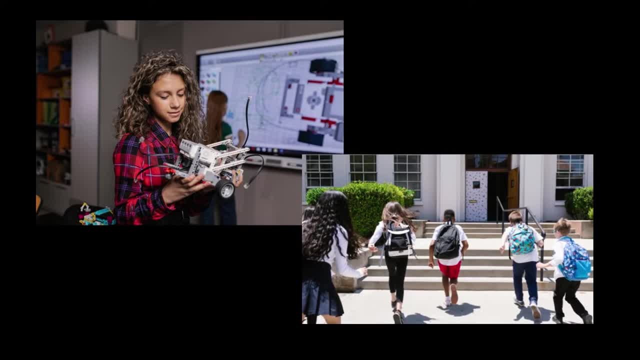 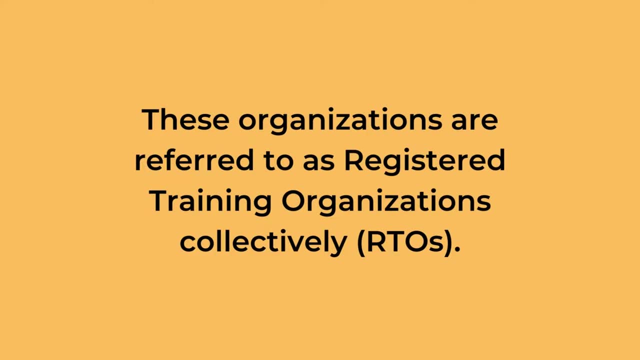 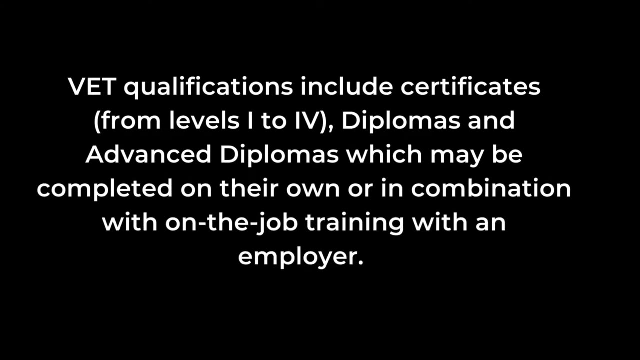 VET courses are also offered as part of the curriculum at some senior secondary schools. These organisations are referred to as Registered Training Organisations, collectively RTOs. VET qualifications include certificates from Levels 1 to 4, diplomas and advanced diplomas. 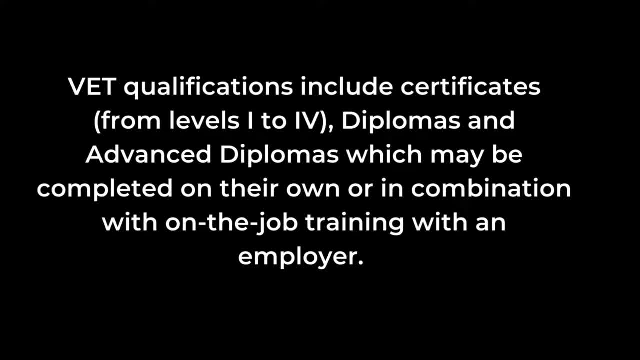 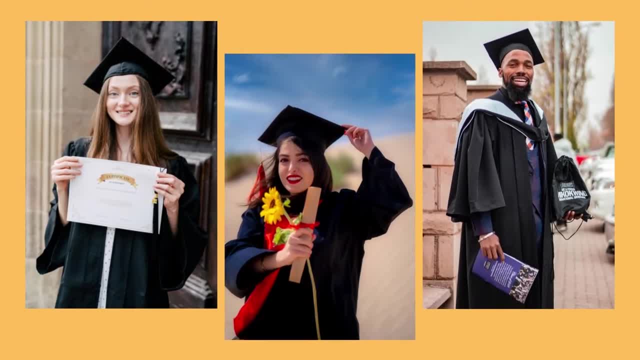 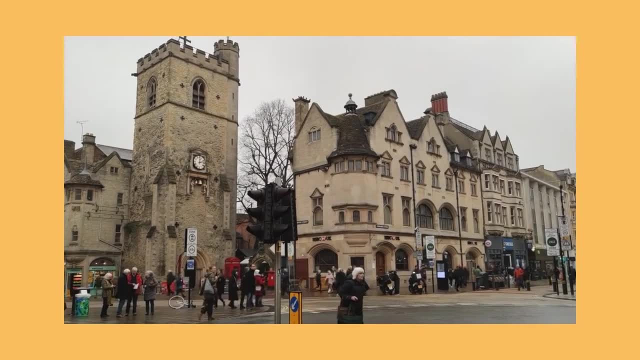 which may be completed on their own or in combination with on-the-job training with an employer. Graduate certificates, graduate diplomas and bachelors can also be earned at some VETs. Technical and Further Education Institutions. Government-funded institutions for vocational education are known as Technical and Further Education TAFE institutes. 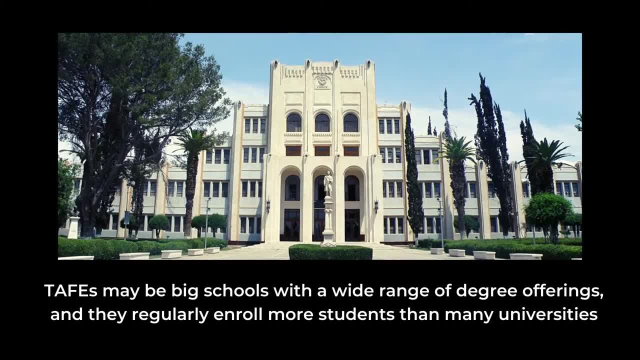 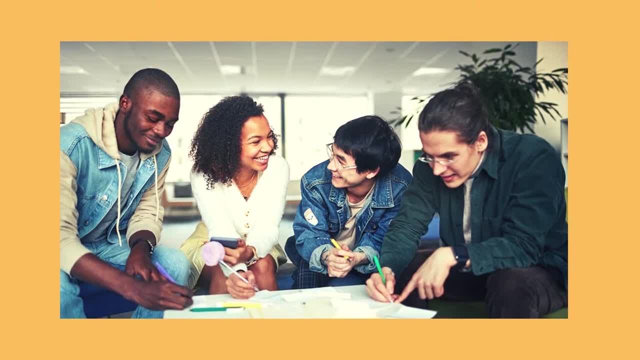 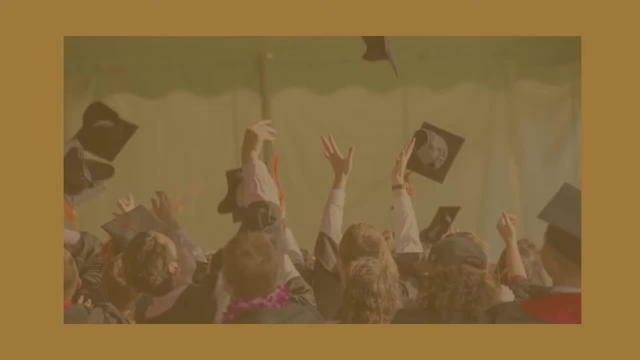 TAFEs may be big schools with a wide range of degrees, and they regularly enrol more students than many universities. The TAFE industry is, in reality, Australia's largest education and training sector. Some TAFEs are associated with universities and can provide bachelor's degrees through the institution. 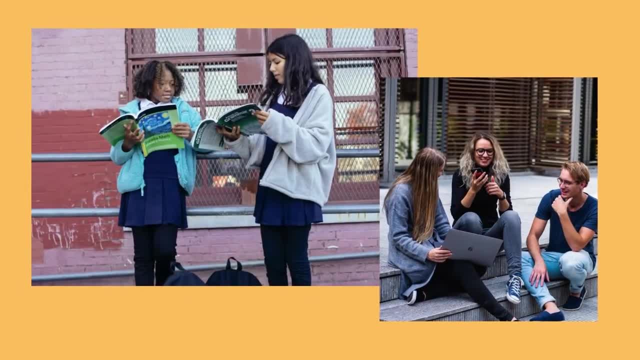 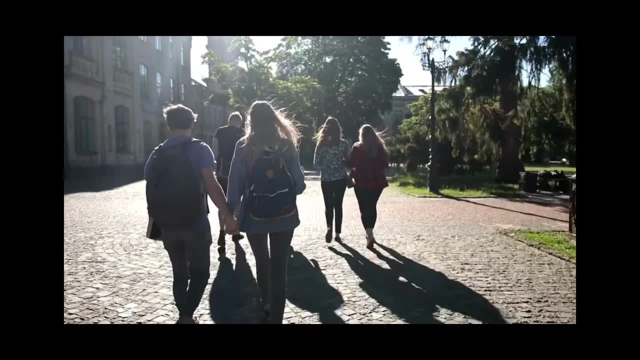 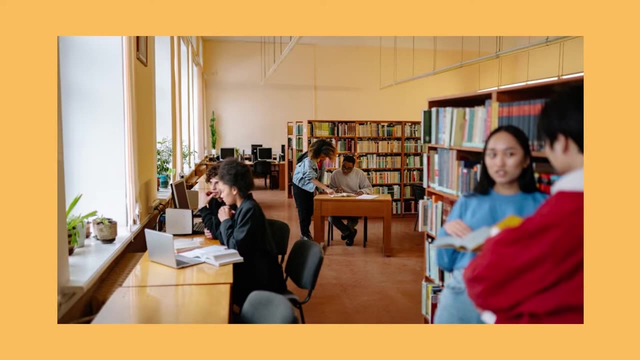 Higher Education. Higher education is a type of post-secondary education that leads to degrees such as bachelor's, master's and doctoral degrees. All Australian universities and a few of VET institutes provide higher education courses. Note that course refers to the course of study that a student decides to pursue in Australia. 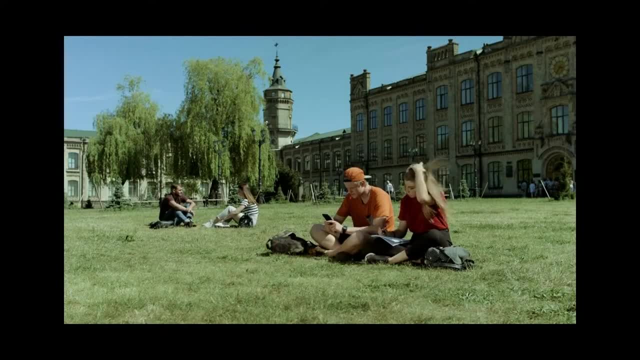 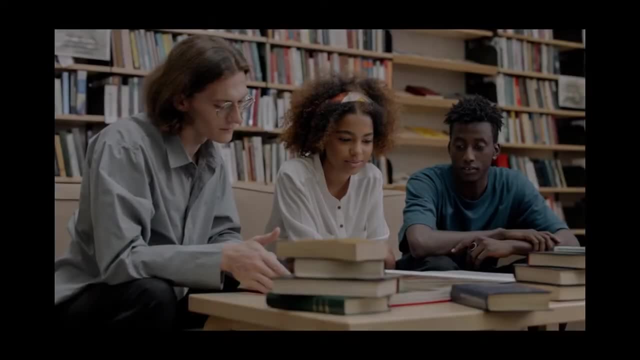 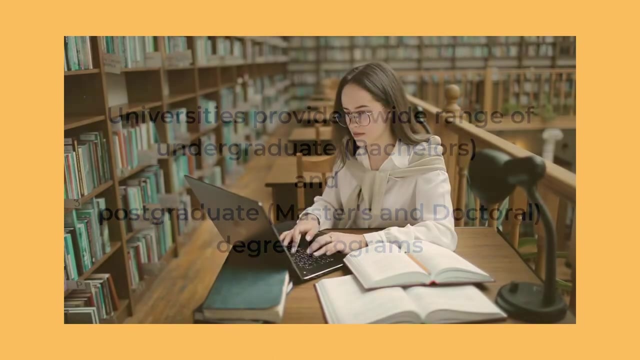 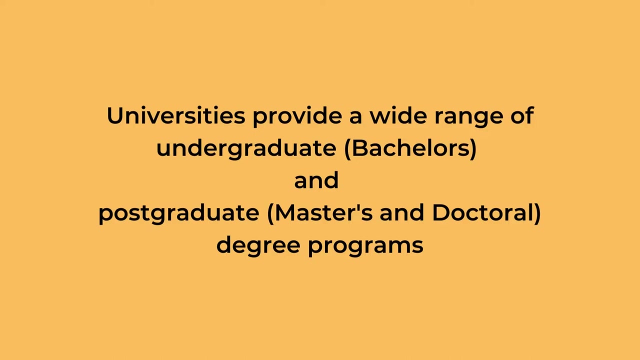 Universities are Australia's principal institutions for higher education institutes- HEIs. In Australia, there are 41 universities, Except for one private and two overseas institutions. all Australian universities are government-funded In all fields of study. universities provide a wide range of undergraduate, bachelor's and postgraduate, master's and doctoral degree programmes. 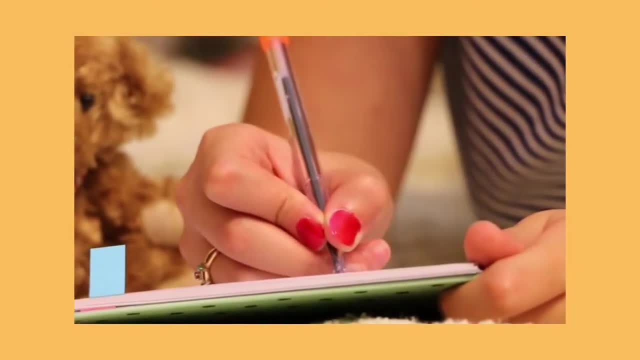 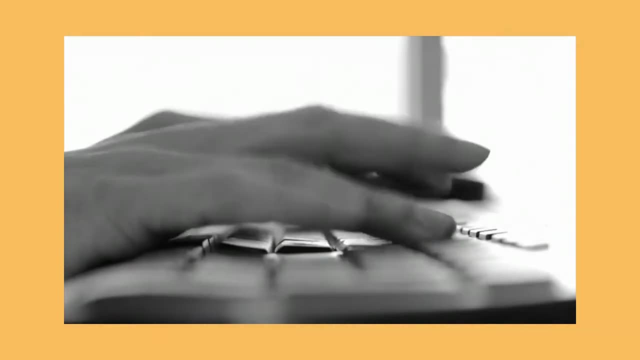 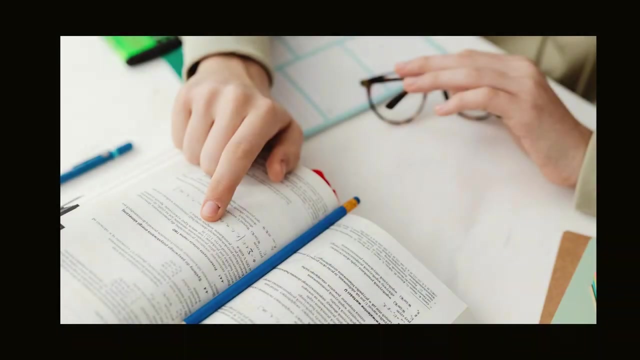 Some universities have dual accreditation, allowing them to provide both VET and higher education programmes. Universities have a more academic focus, with heavy emphasis on essay writing and exams. Students get much deeper knowledge of the field or subject matter they are studying. They are often referred to as their chosen major or area of specialisation. 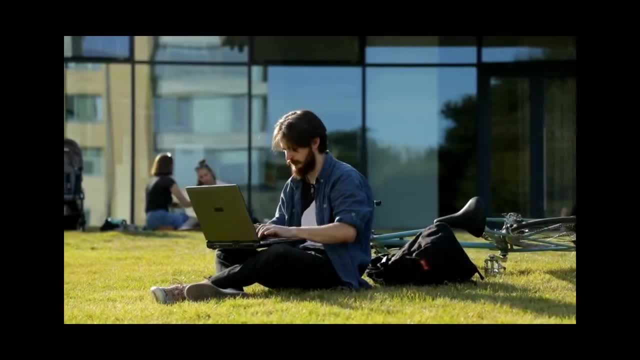 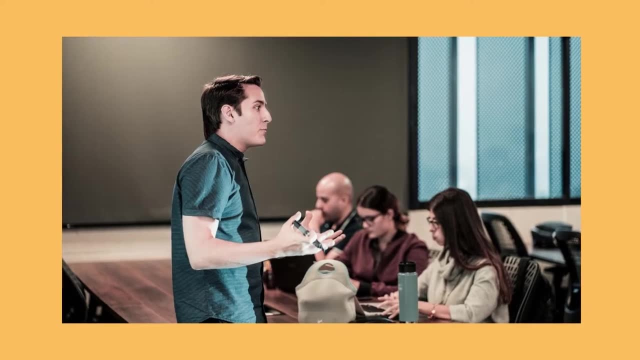 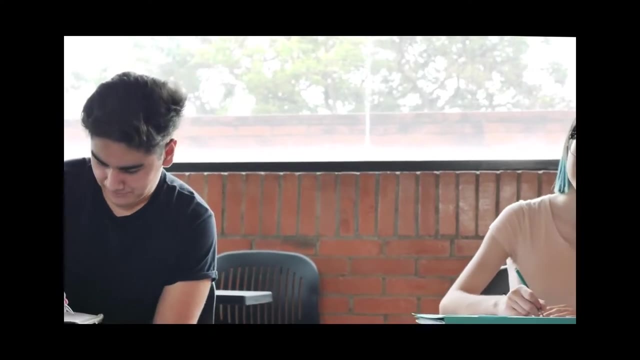 They also strengthen their personal attributes, developing professional and transferable skills, rather than focusing only on industry-specific occupational skills. Due to the in-depth curriculum, undergraduate university courses are typically three or four years long, resulting in bachelor and honours bachelor degrees. Some universities also offer two-year associate bachelor degrees. 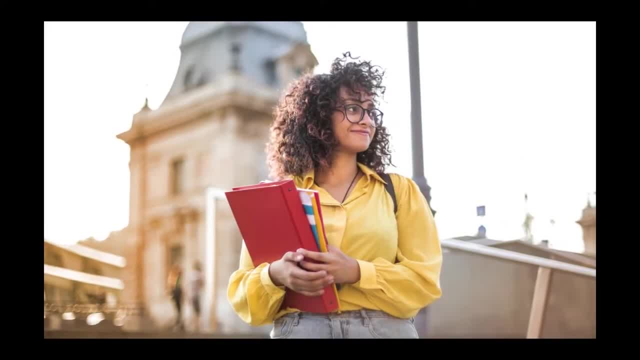 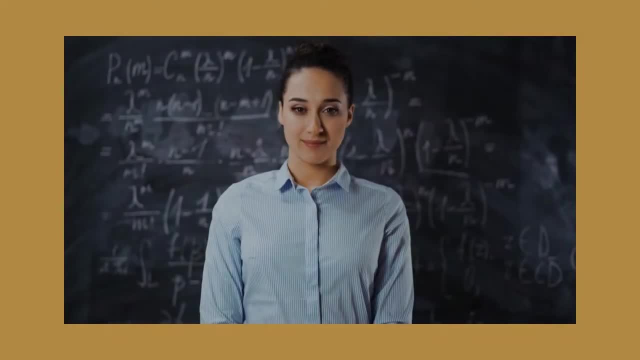 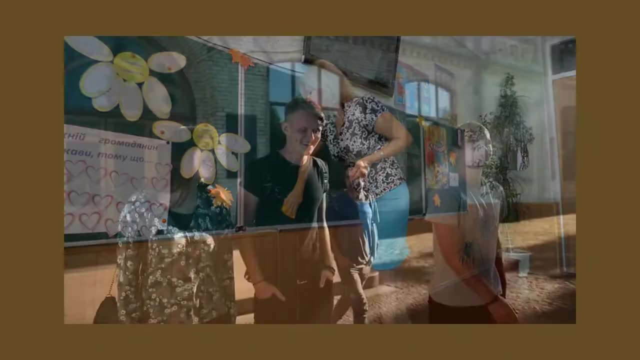 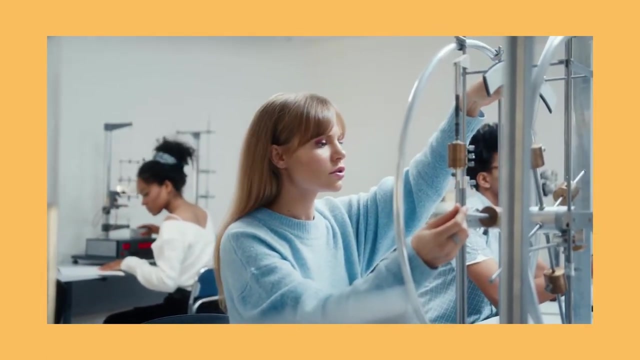 courses or programs. a bachelor degree is typically required for acceptance into professional programs such as medicine or law, as well as for academic jobs, research based careers and professional roles like engineering or teaching. a bachelor degree is also required to pursue any postgraduate degrees, which can be a study based or research based master, followed by a doctorate degree. 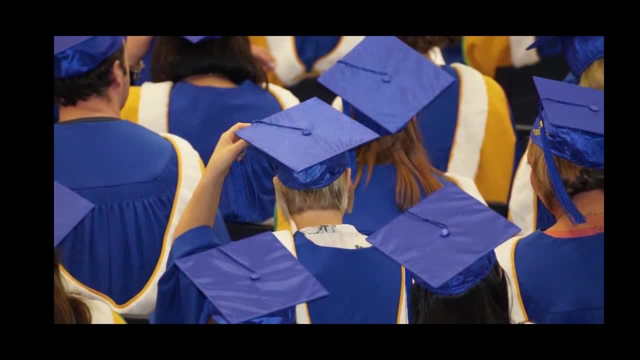 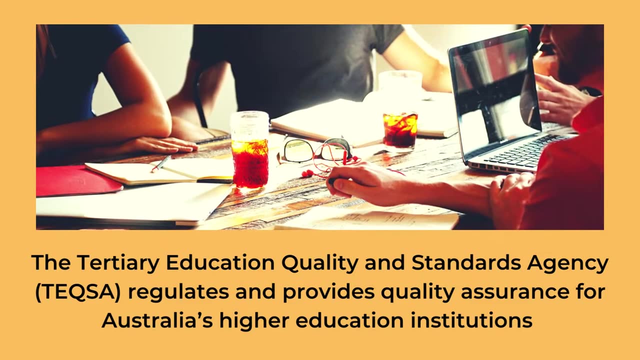 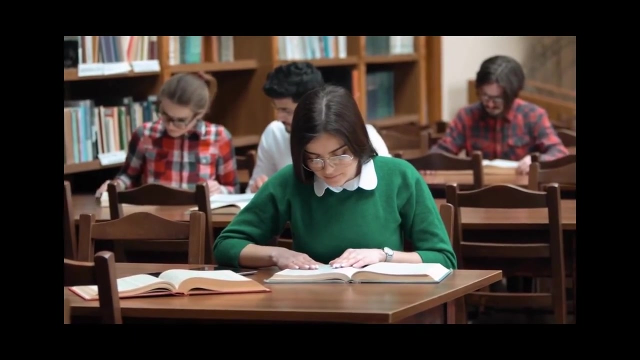 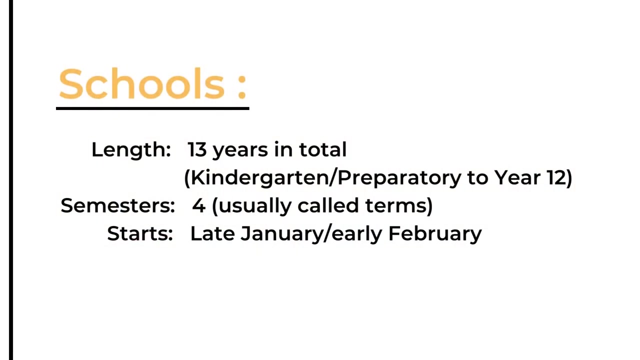 which is the highest level of academic standing students can achieve. the tertiary education quality and standards agency, TEQSO, regulates and provides quality assurance for Australia's higher education institutions to ensure students get the same high caliber of education regardless of where they study. schools length 13 years in total: kindergarten or preparatory to year 12. 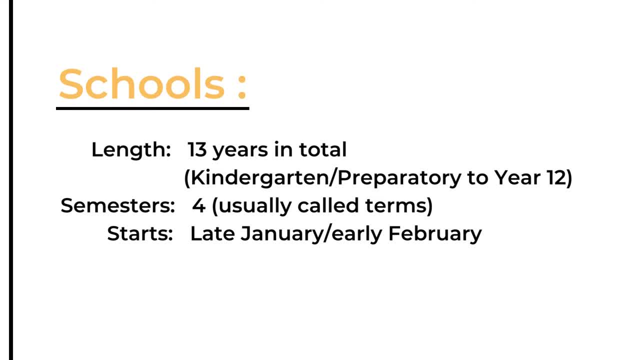 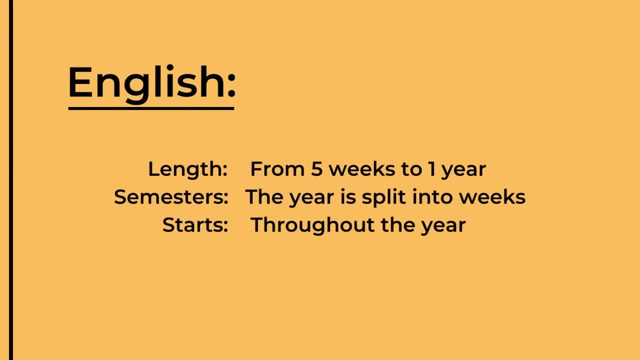 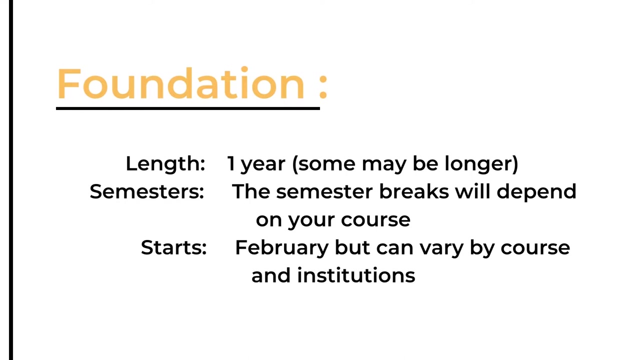 semesters, usually called terms. starts late January or early February. English length: from five weeks to one year semesters: the year is split into weeks. starts throughout the year. foundation length: one year. some may be longer semesters: the semester breaks will depend on your course. starts February but can vary by 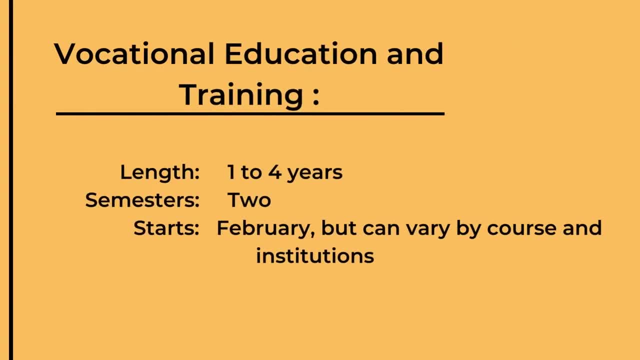 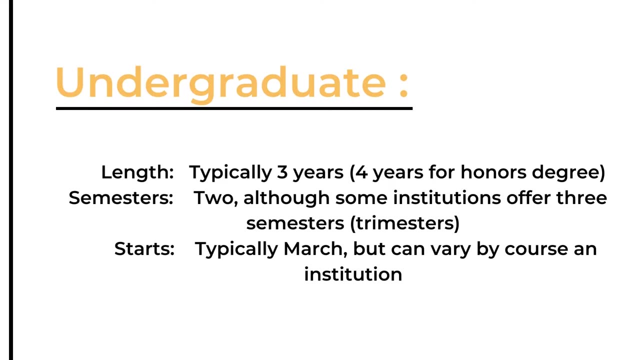 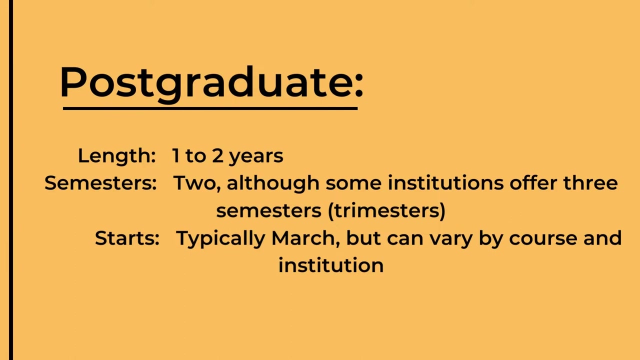 course and institutions. vocational education and training length: one to four years. semesters to: starts February, but can vary by course and institutions. undergraduate length: typically three years, four years for honors degree. semesters to, although some institutions offer three semesters. trimesters starts typically March, but can vary by course and institution. postgraduate length: one to 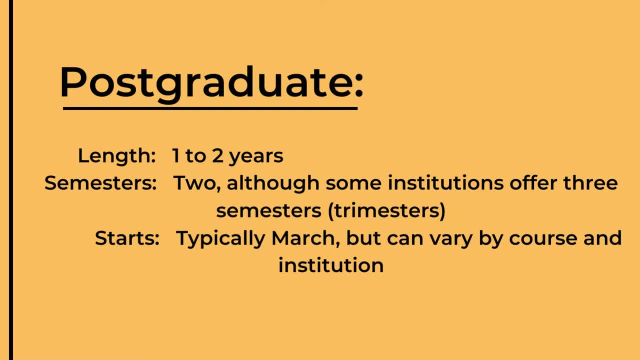 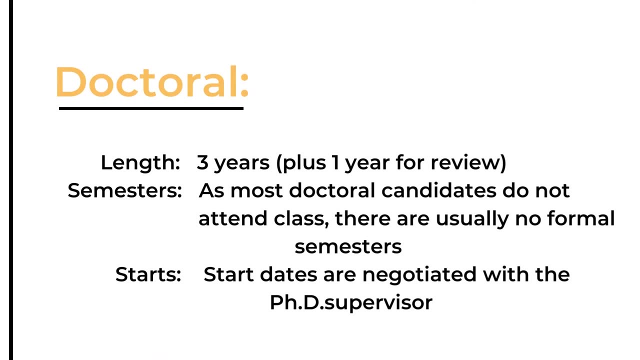 two years semesters to, although some institutions offer three semesters. trimesters starts typically March, but can vary by course and institution. doctoral length: three years plus one year for review semesters. three years plus one year for review Semesters. As most doctoral candidates do not attend class, there are usually no formal semesters. 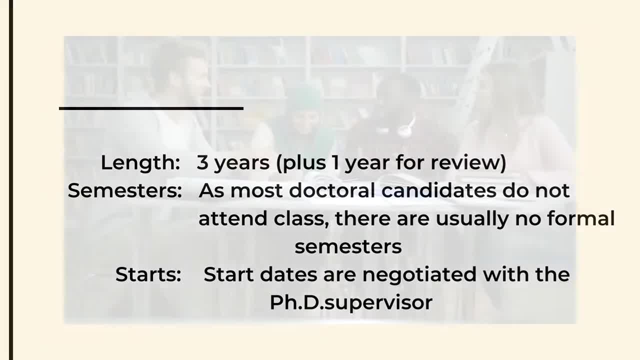 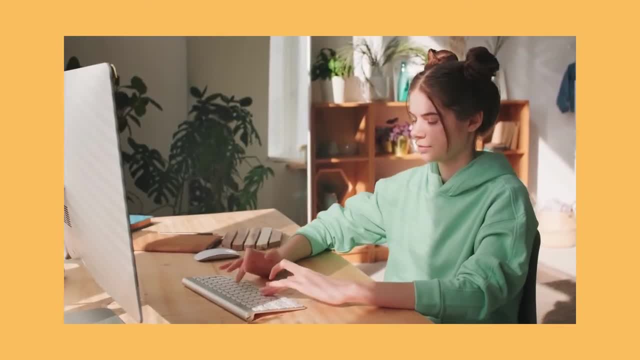 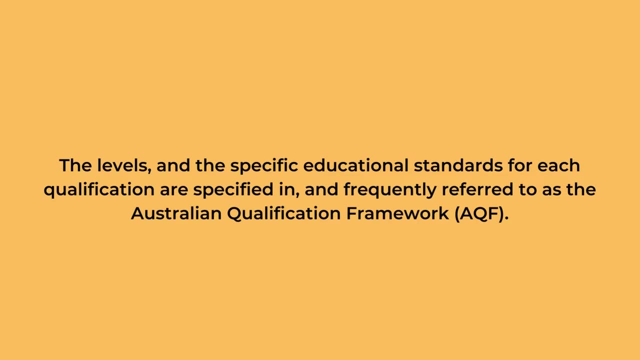 Starts. Start dates are negotiated with PhD supervisor. There are 10 levels of qualifications that students can earn in Australia after completing their school education. The levels and the specific educational standards for each qualification are specified in, and frequently referred to as, the Australian Qualification Framework, AQF. 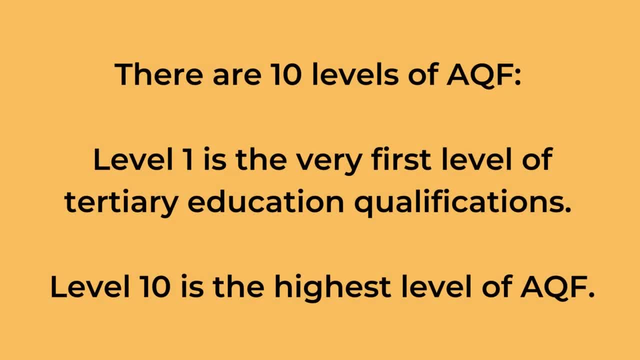 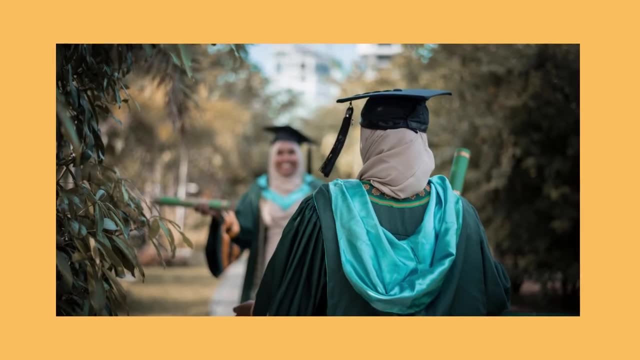 Levels of qualifications. There are 10 levels of AQF. Level 1 is the very first level of tertiary education qualifications. Level 10 is the highest level of AQF matched to the highest level of education. a student can achieve A doctorate degree. Types of qualifications. 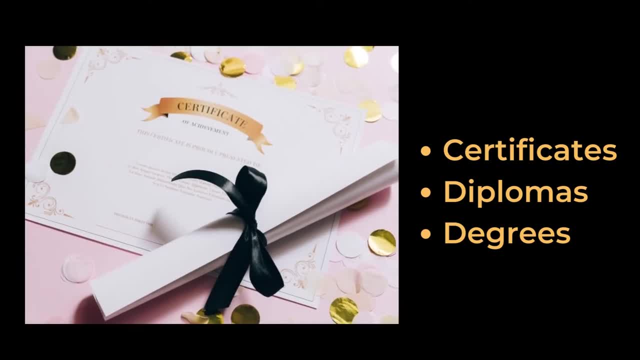 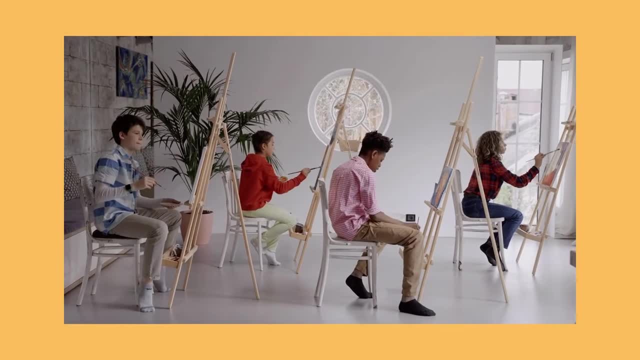 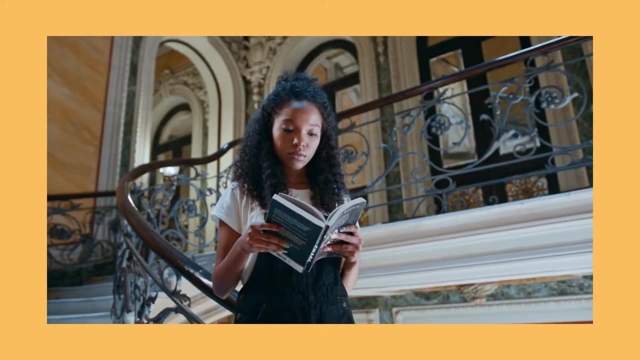 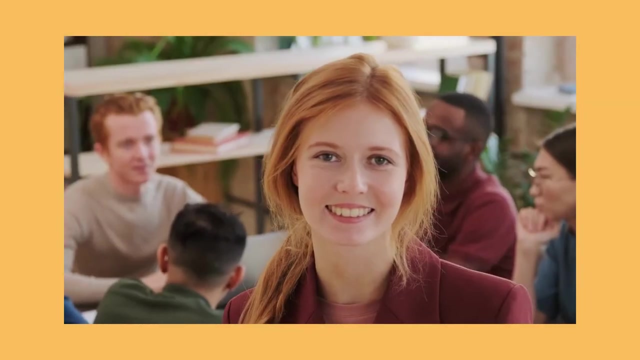 The various different qualifications That a student can achieve in Australia can be grouped into certificates, diplomas and degrees Certificates: Certificate courses are offered in schools and VETs, Ranging from 6 months to 2 years in duration. These courses provide introductory skills and training, delivering industry-specific knowledge and skills in communication, literacy and numeracy, and teamwork. 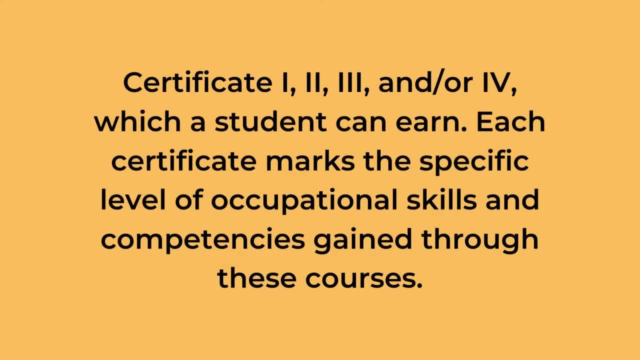 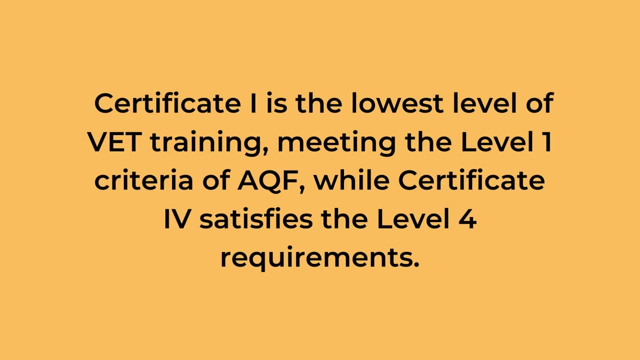 There are four distinct certificates- Certificate 1., 2., 3. And or 4,- which a student can earn. Each certificate marks the specific level of occupational skills and competencies gained through these courses. Certificate 1 is the lowest level of VET training, meeting the level 1 criteria of AQF. 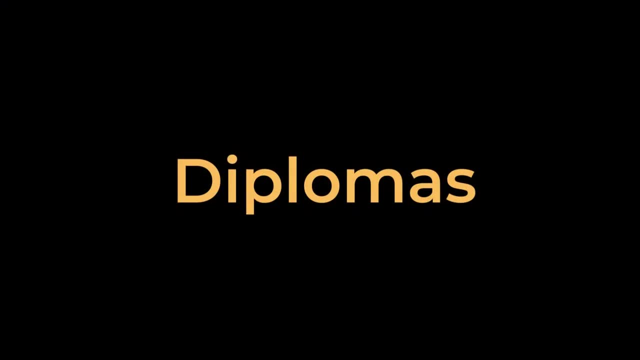 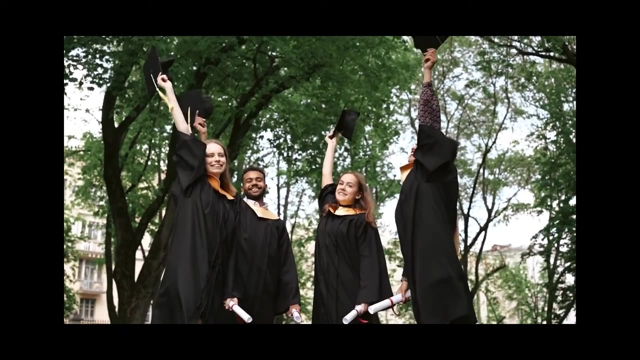 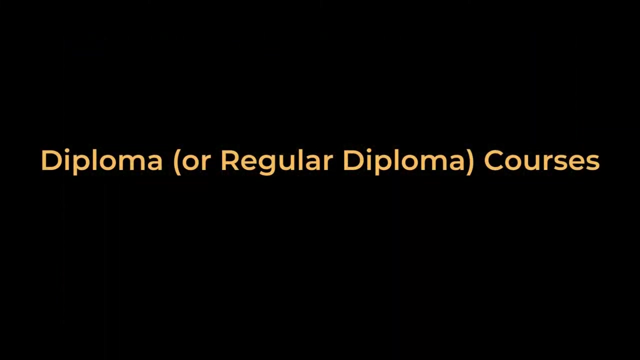 While Certificate 4 satisfies the level 4 requirements, Diplomas. Diplomas can be earned in vocational education and training and in some higher education institutes. Diplomas fall into three sub-categories: Diploma or regular diploma Courses Prepare students for industry, enterprise and paraprofessional careers. 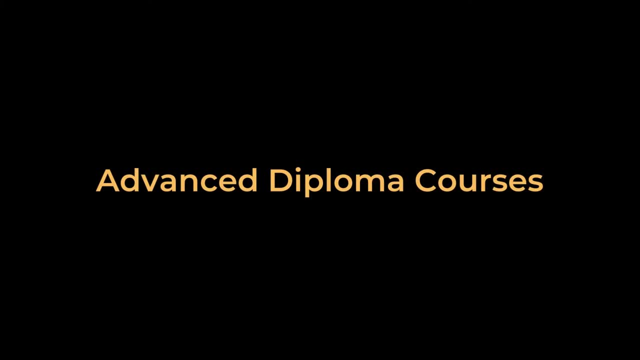 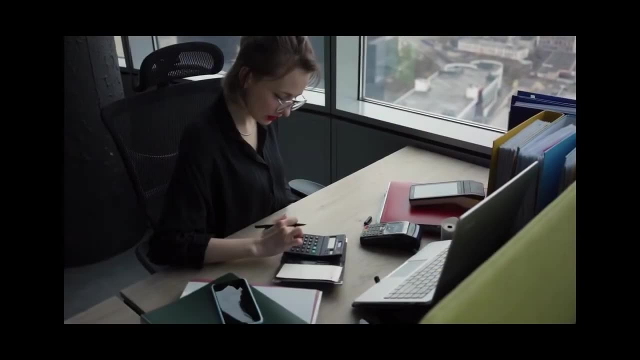 Diplomas typically require 18 months to two years of full-time study. Advanced Diploma Courses Provide a high level of practical skills for advanced skilled or paraprofessional work in areas such as accounting, building design and engineering. Students can complete some advanced skilled or paraprofessional work in areas such as accounting, building design and engineering. 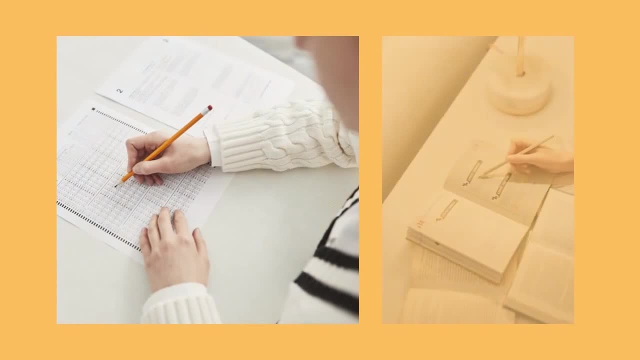 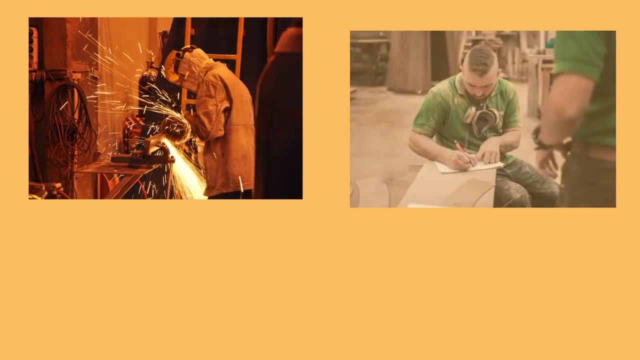 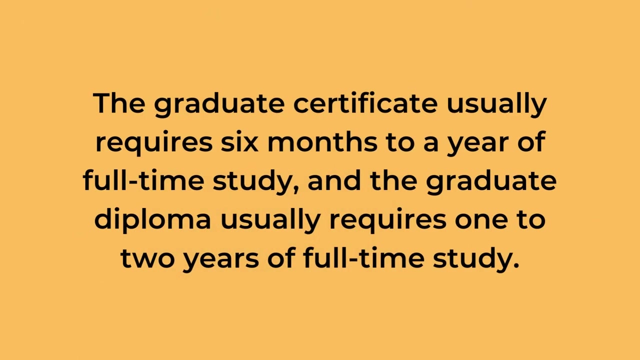 some advanced diploma courses at university level. Advanced diplomas vary in length, from two to three years of full-time study. Graduate certificate and diploma courses provide high-level employment-related skills and knowledge. The graduate certificate usually requires six months to a year of full-time study and the graduate diploma usually requires one to two years of.